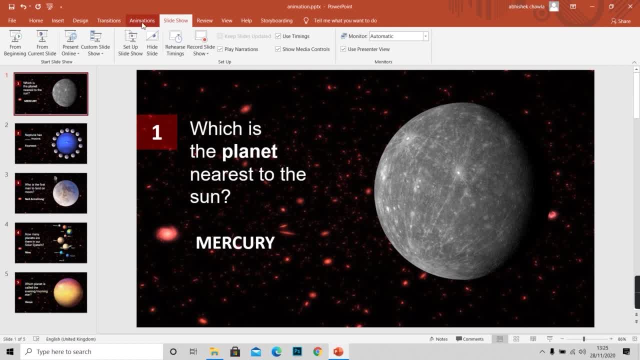 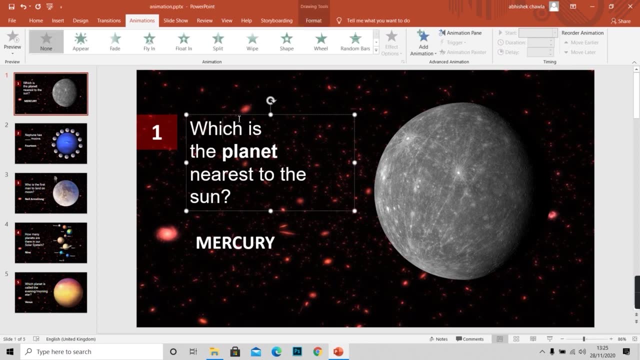 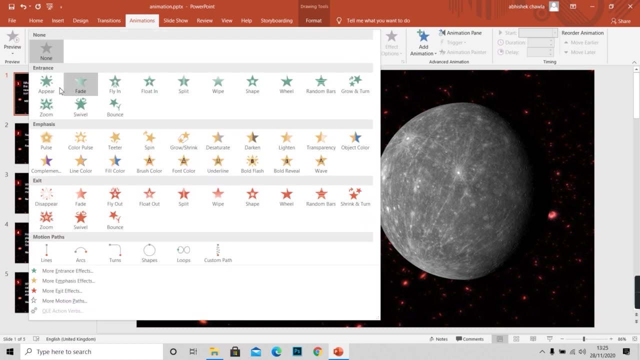 For that we have this menu item here, menu tab here, animations. We will click on it and we will select the object, the item that we want to be get animated. For example, I will select the text here, Okay, And I will choose the animation from here. These animations work when an object enters. 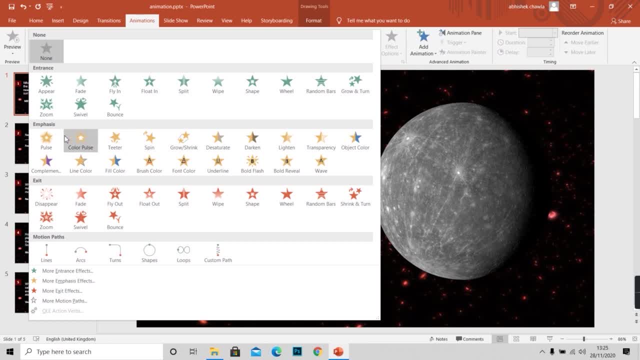 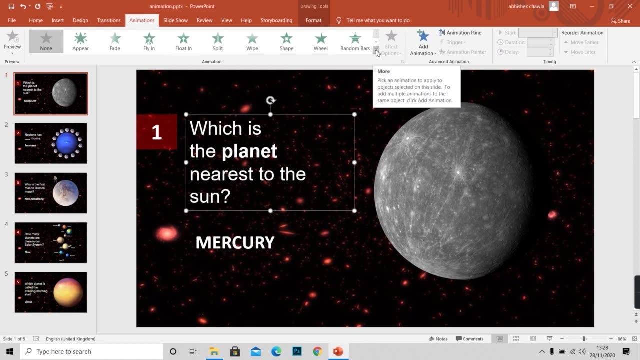 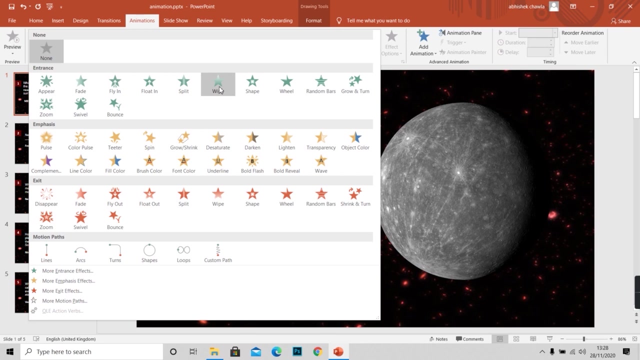 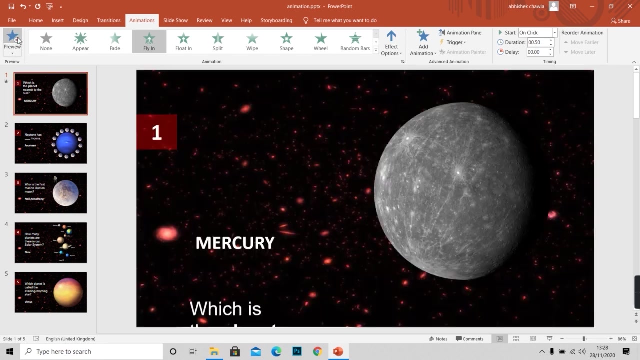 a slide. These animations work when an object is on the slide And these are the animations that will work when an object exits the slide. So we will select the object first and then I will select the kind of animation that I want. For example, in the entrance I will want this, maybe fly-in. You can see the preview. 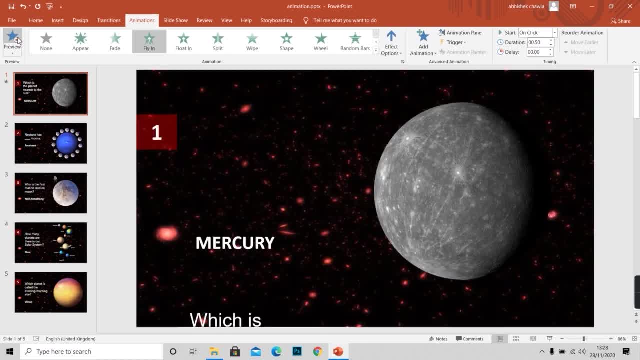 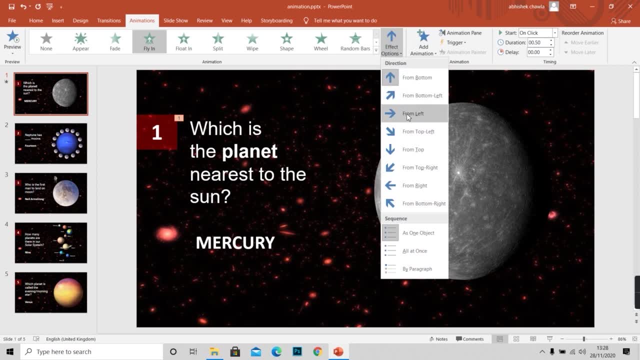 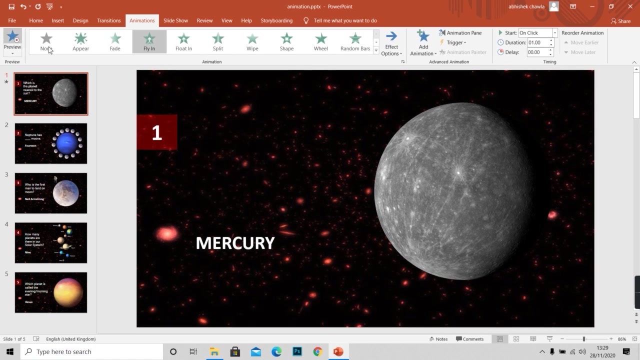 from here. I can even change the direction effect options. I want it from left like this: If you want the animation to get slowed down, Okay, This is the duration that I am changing from 0.50 to 1.. Now I will see the result. 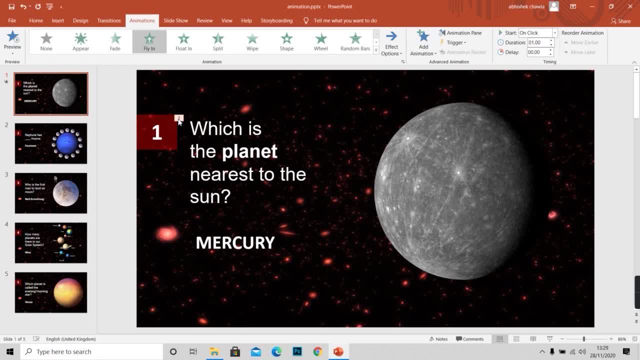 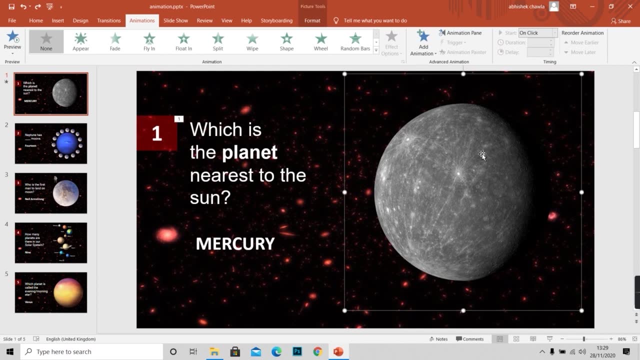 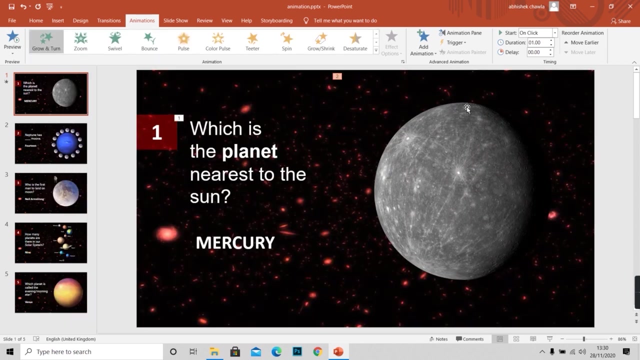 You can see 1 is written here. That is. this is the animation actually. If you want to delete this animation, you will select this one And press delete. Next I want to animate this Mercury planet image here. Here I will choose, grow and turn. 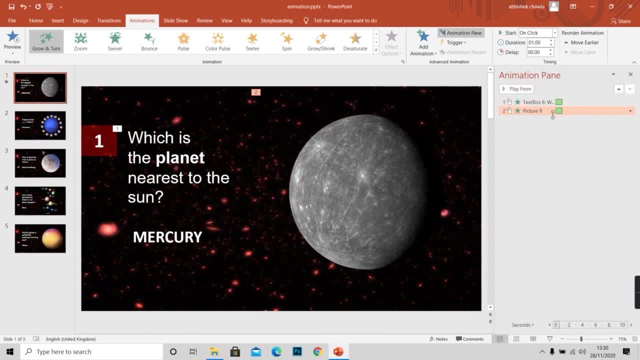 I will go to animation pane here. This is the panel basically that controls the animation. I will say It says on-click, That means when I click the mouse button the animation will proceed, But I want it after the previous animation, So I will select it after previous. 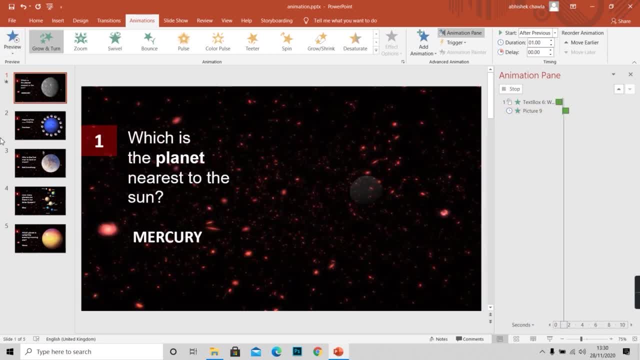 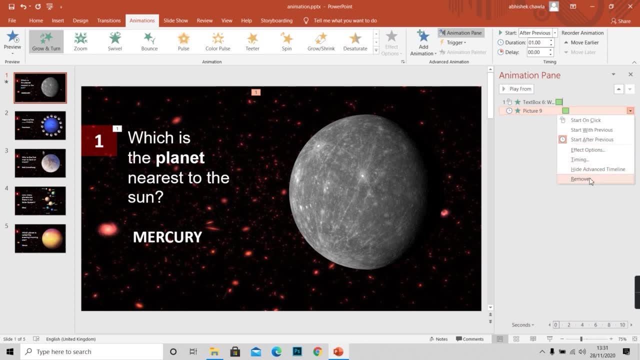 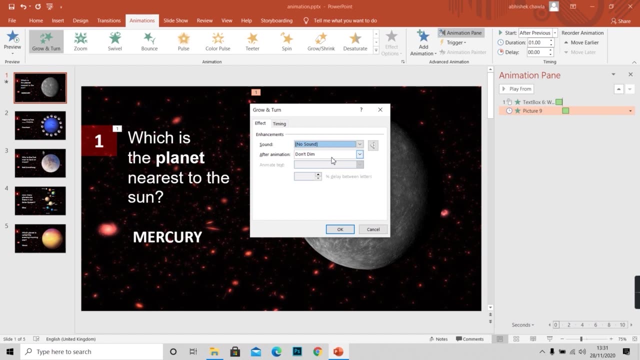 Now, if I see the preview, Its working automatically. We have more options here. Okay, here, like, if I go to effect, you can give sound after animation, don't dim. next is our timing, like if I want to repeat, yes, I want it repeat, maybe until next click. 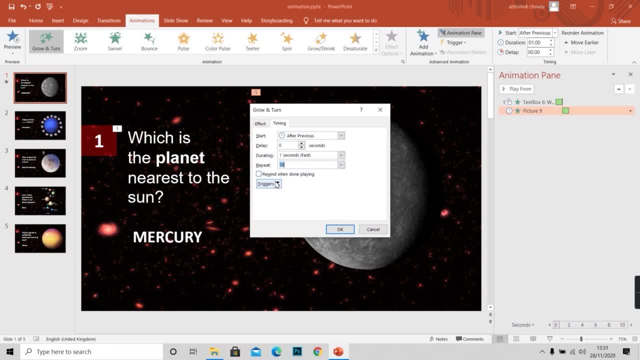 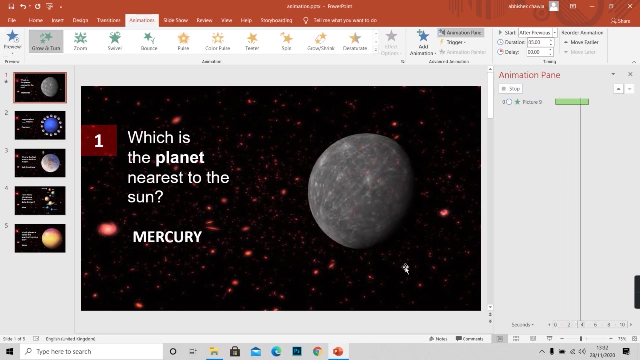 or maybe 10 times. okay, if I say okay, this will happen. I wanted to get delayed maybe five seconds. the whole animation will take place in five seconds here. I'll press ok and we'll see the result. this is absolutely what I want. now I'll go to this. 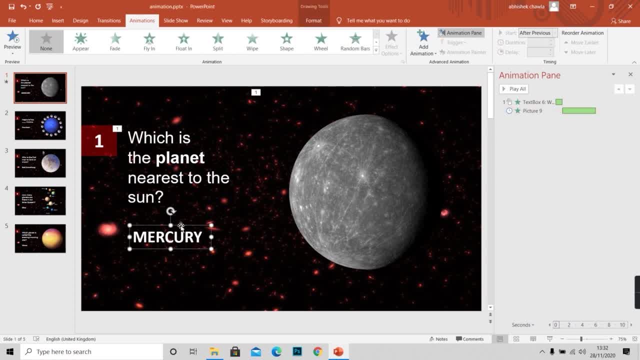 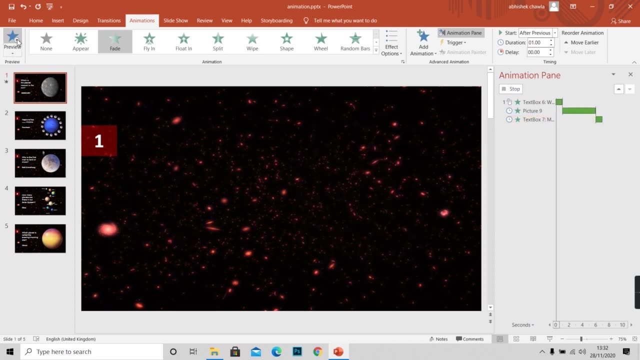 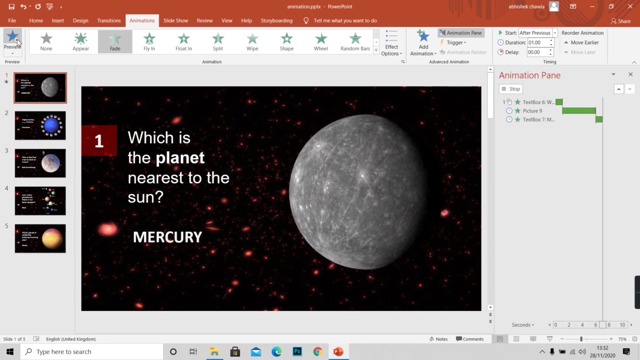 text here. that is the answer of our question and I'll select fade after previous duration and I'll see the preview. the question comes first, then the image, then the answer. I am animating the image after the question just because I want to give the audience some time so that they can. 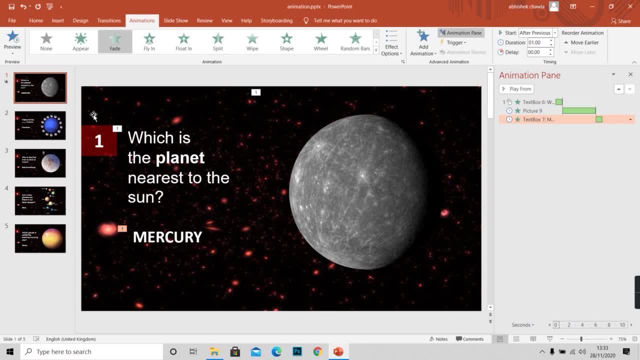 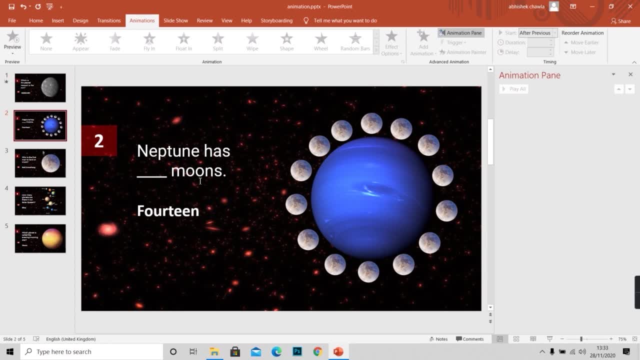 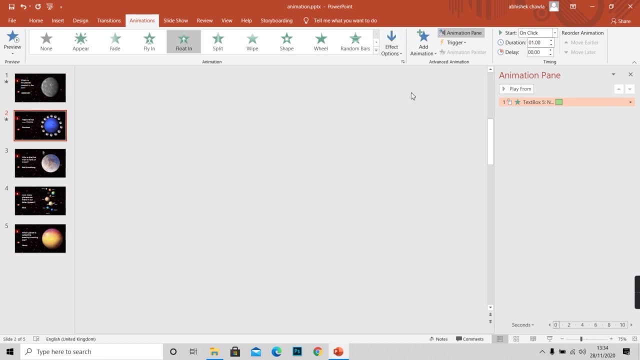 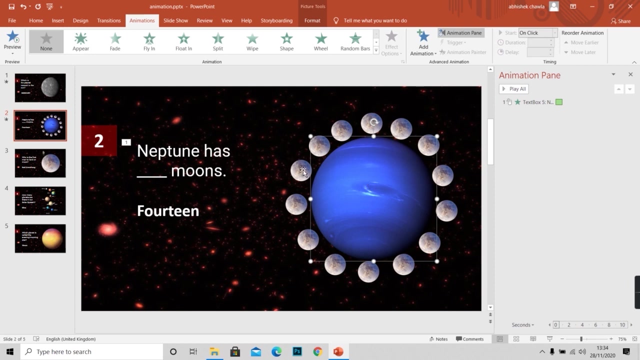 think about the answer. next we'll go to our next slide. here we have: this is the question, this is our answer and this is the image. let's select the object. this time I will select float in, then I'll have this image here. first of all, I want this after previous. this is: 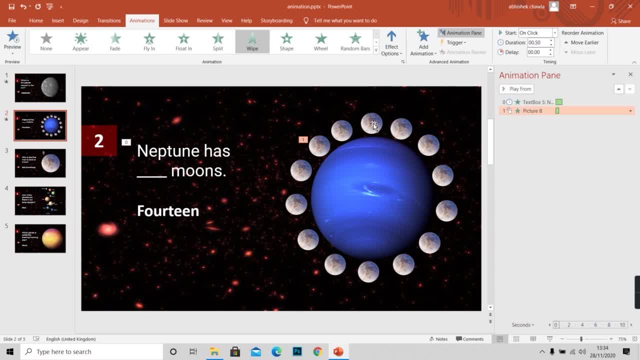 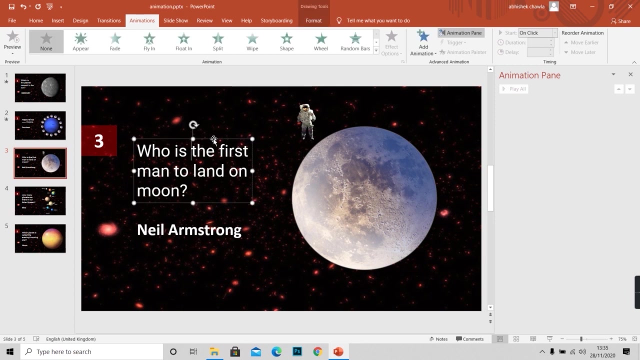 the image here of the Neptune, or I can even have this deleted and I'll only animate these 14 moons here. I'll select them all, moon them after previous. that is okay, and then I will select the answer here. as you can see, it is very easy to give some kind of animations to your objects. 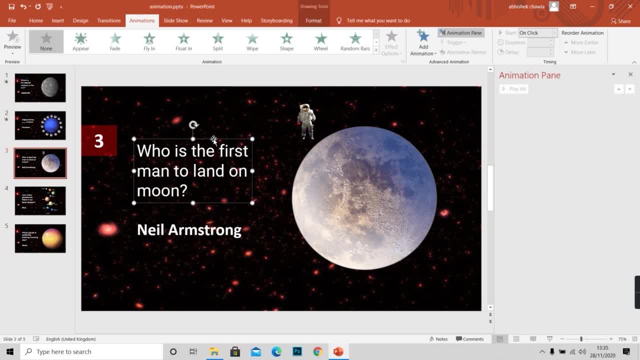 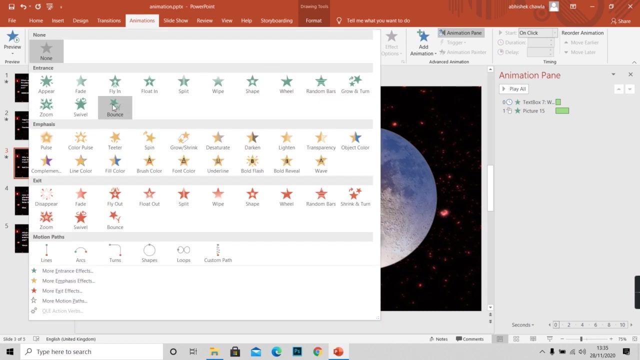 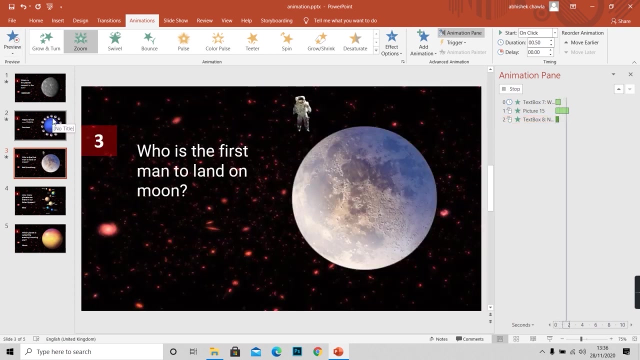 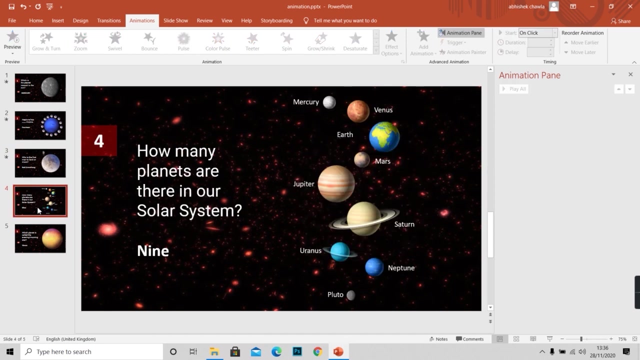 in PowerPoint. this is the basic animation tutorial. again, I'll select the objects, the animation that I want. when I want it to be done, maybe I will give it bounce, okay and then ok. so this is our slide. this looks quite cool. this is our fourth slide. the question then: I want this. 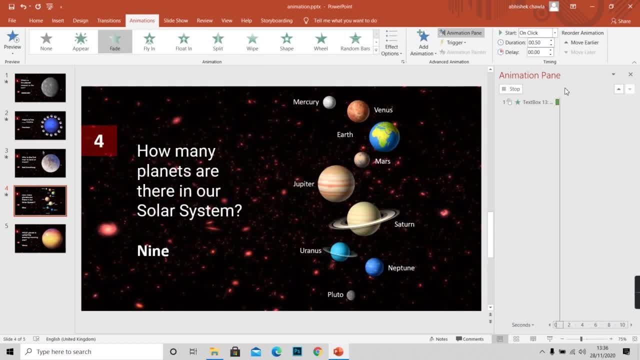 the question, then I want this, but after previous. this will also after previous. again, I'll give it fade after previous. what I want? these namesádE we'd after previous fade beis editing. we'll take a break after previous. I want these names to get displayed one by one. that is what I am doing here.